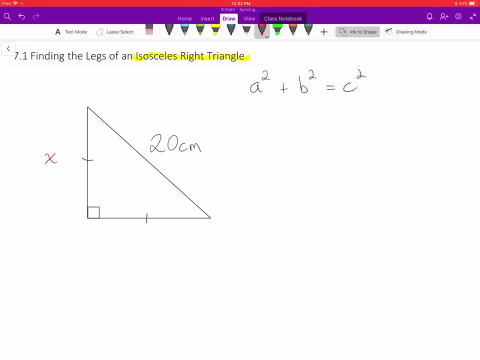 So they can be represented with the same variable. So in this case, that could be x and that could be x. So, with that being said, we could actually find the value of x using Pythagorean Theorem And as we're doing that, it looks a little bit different than when we have two sides given and we're asked to find the third. 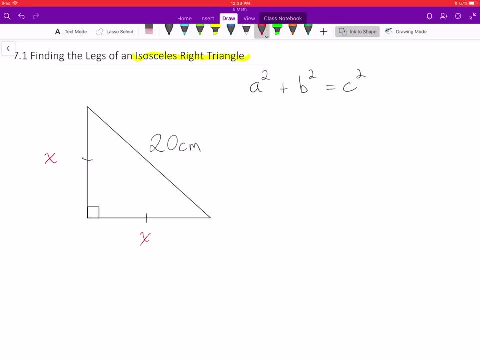 But it can still be different. So I would ask: if you guys really haven't seen this before, why don't you hit pause and try it on your own, See if you can figure it out? You might actually surprise yourself. And then hit, play and kind of see how I'll demonstrate a strategy that you can use and a way you can have it kind of written to show what you're thinking. 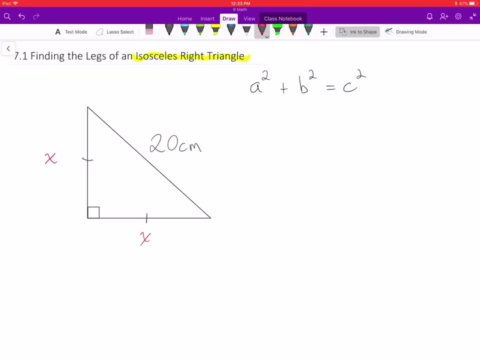 So go ahead and try to hit pause, Try it on your own And then hit, play and see what you get, All right. So once you've tried this on your own, this is how I would probably do this. I would probably do this and show my work. 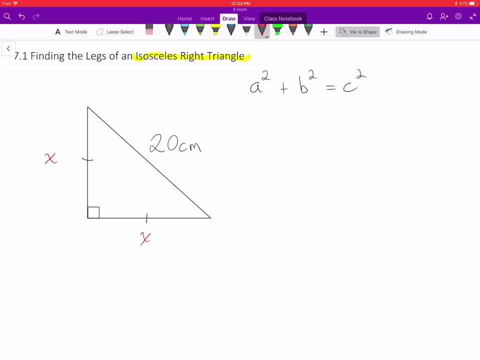 If you want to kind of mimic the way I do this, as long as it makes sense for you, that's fine too. So I know that some of my legs squared, a squared plus b squared, has to equal c squared, So I can identify all three sides. 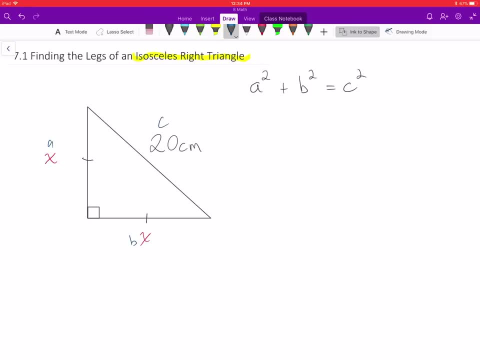 So obviously the two legs are a and b. c is going to be that hypotenuse, which is 20.. So a squared would have to be x squared And I would have to add that Again with another x squared And that would have to equal 20 squared. 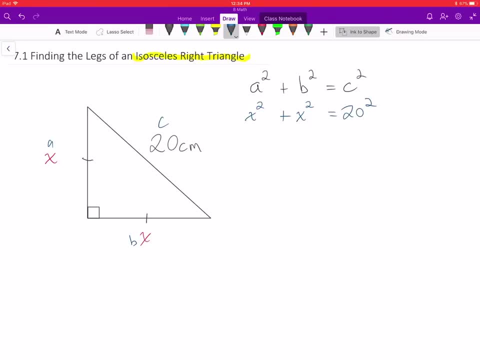 Well, since I still have the same variable in this entire equation, it is still solvable, Because these two x squareds are like terms, so I could actually combine them together. When you're adding two things that are the same, you have two times that thing. 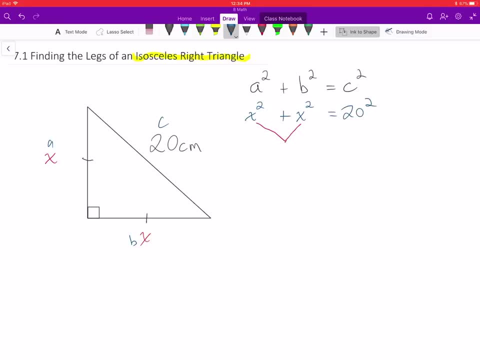 So since I have two x squareds, or x squared two times, I can write that as two times x squared And 20 squared would be 400.. So what I'm working with now is I have two times x, squared is 400.. 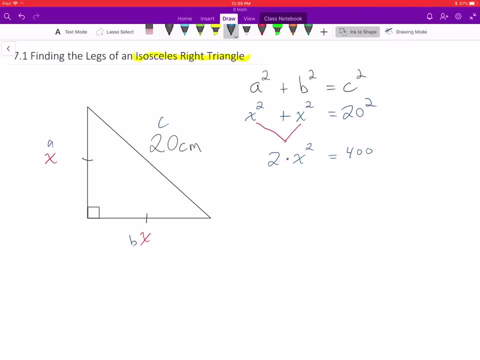 I can isolate the x squared piece by dividing both sides of the equation by two. All right, If I had two x squareds as 400, a single x squared is what I would have left- should equal 200.. So that x squared equals 200.. 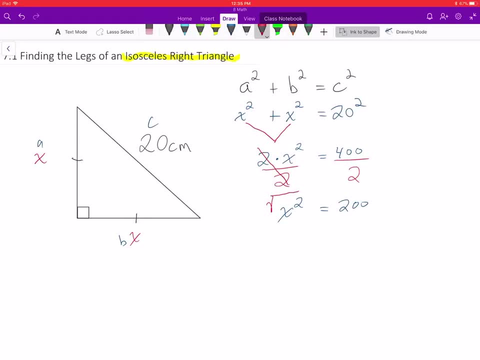 I can then take the square root on both sides of my equation, The x squared is canceled out, leaving with just x. And then the square root of 200 would be the exact answer, because 200 is not a perfect square. There is not a whole number that would multiply by itself to make 200.. 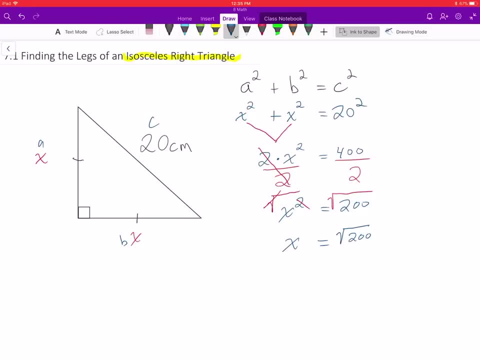 If I were to ask for an approximation or we wanted to have some sort of an approximation for this and we could really round it to any number we want or, I assume, any place value we want. I'm going to just round this to the nearest tenth. 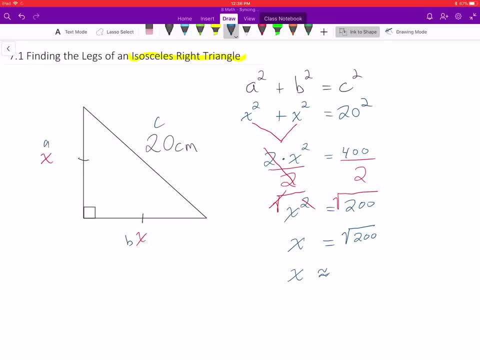 And I have in the calculator 14.14213562.. The number in the tenths place is a 1.. The number after that is a 4.. That's going to tell me to round down to 14.1.. So I should have 14.1 for this one. 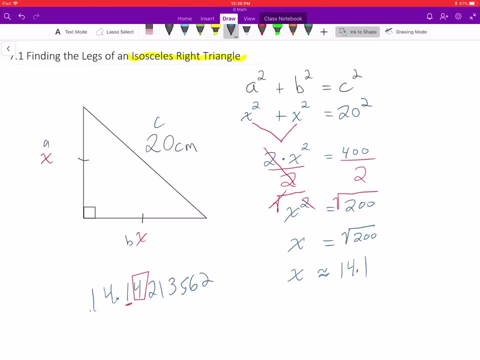 So I know that this distance on both sides will be 14.1 as my approximation. If I want to check my answer- and this is very important- if you're checking your answer, try using the exact answer Which, as we kind of look back here. let me do this. I'm going to circle here. 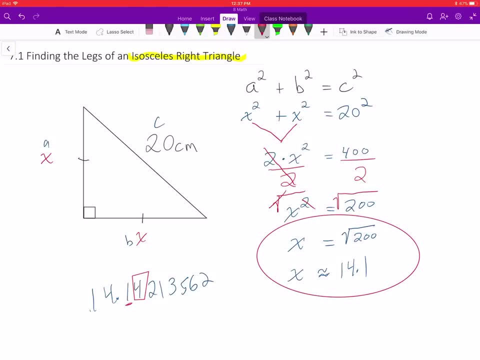 Those are my two different answers. I have an exact answer and I have an approximate answer. The exact answer is the square root of 200.. I did not round that at all. The approximate answer is the 14.1.. I had to round that and I rounded it down. 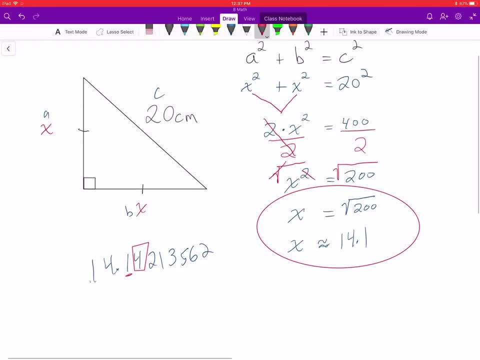 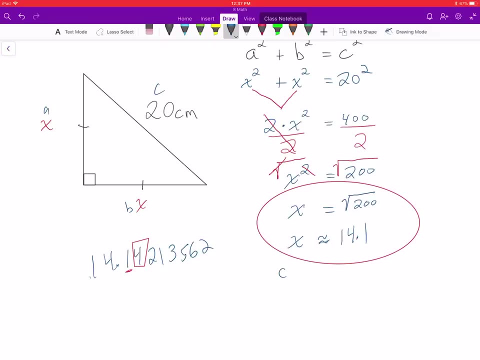 So it's actually a little bit smaller than the actual answer When I'm checking. so say, I want to do a check, which is always helpful to do. I'm going to check. I'm going to plug all three numbers back into the Pythagorean theorem.